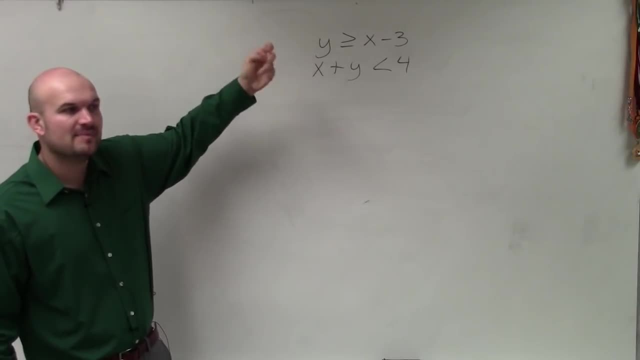 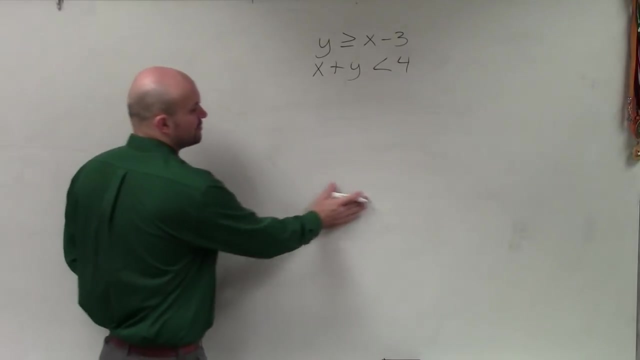 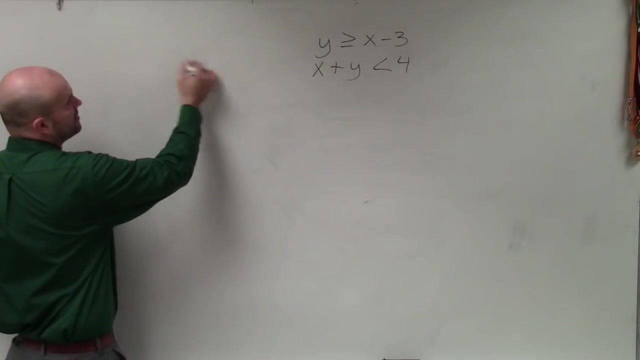 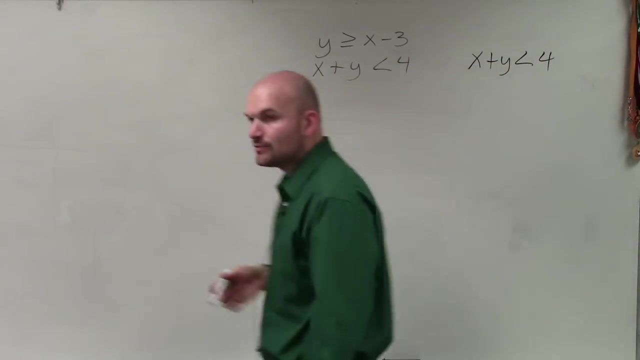 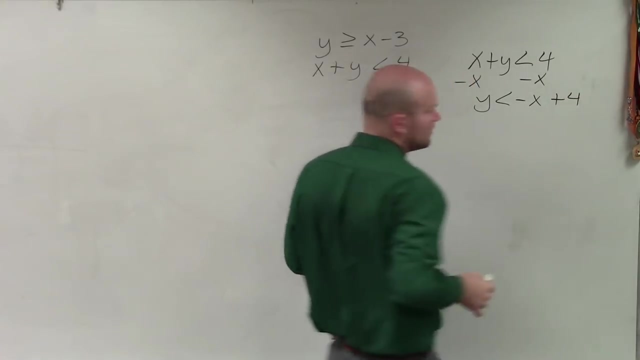 to incorporate it in with the rest of the lesson that we're going to be talking about today. negative x plus 4.. Now, remember, when graphing with a negative 1 as your slope, when you have a negative x, remember we need to have a number. 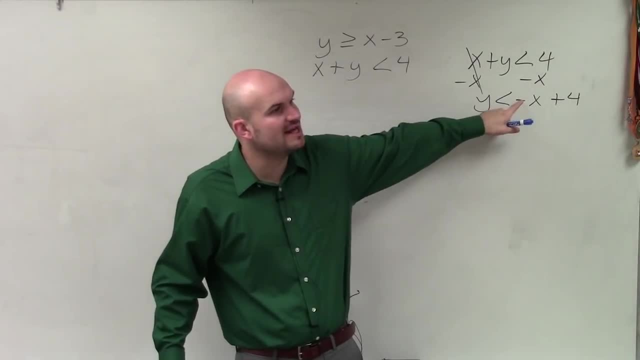 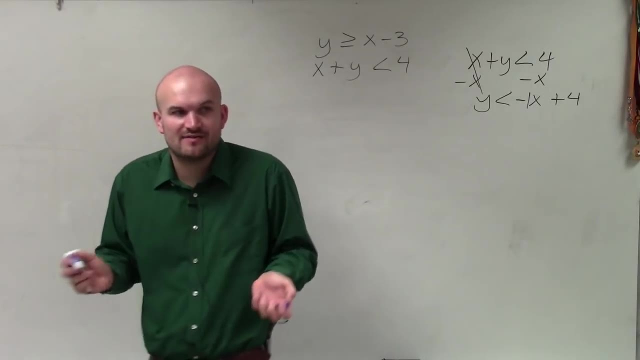 We need to have a fraction as our slope, So our coefficient. you have the negative. Remember we can always write in that's a negative 1.. That doesn't change the problem. Negative 1 times x is just negative x. But again, remember I said I always. 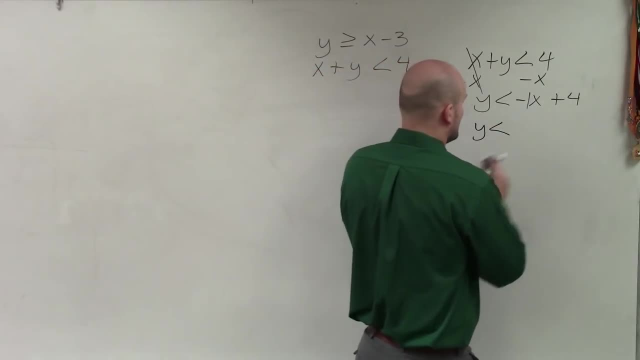 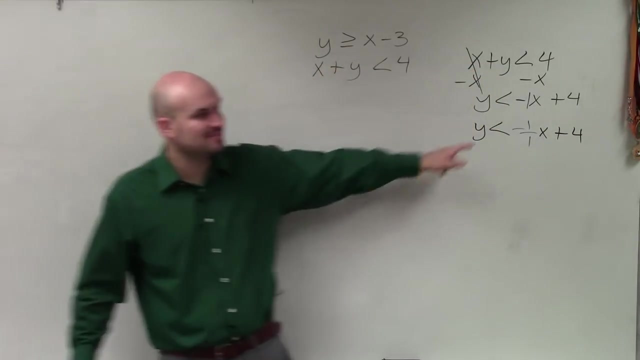 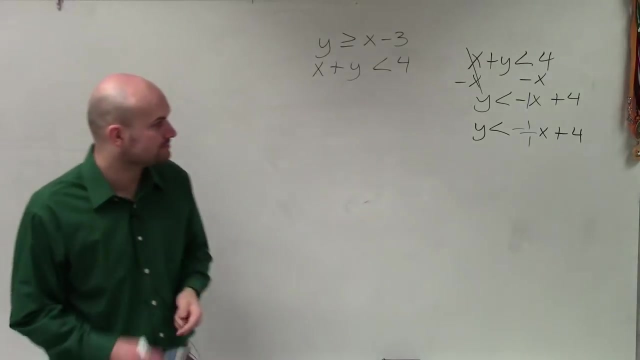 want to have it as a fraction, So I'm going to write this over 1.. Because negative 1 divided by 1 is the same thing as just negative 1.. But when I'm computing my slope, I like to be able to use fractions with that. 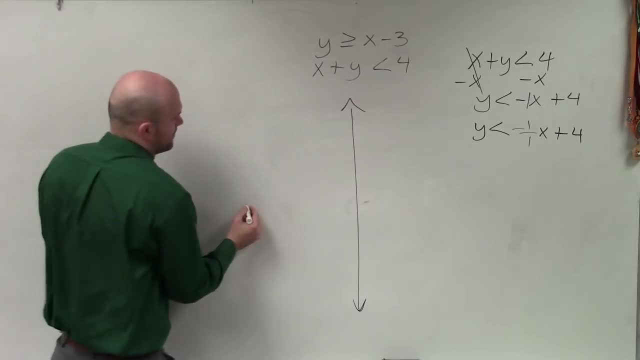 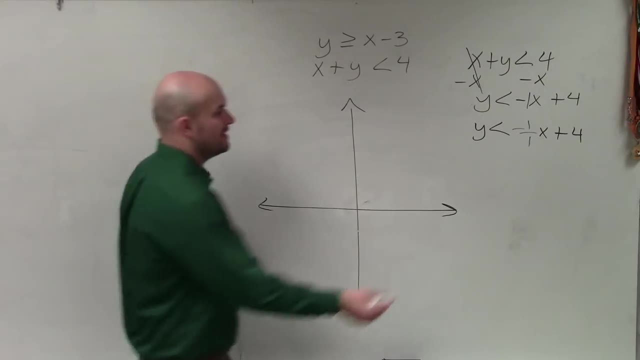 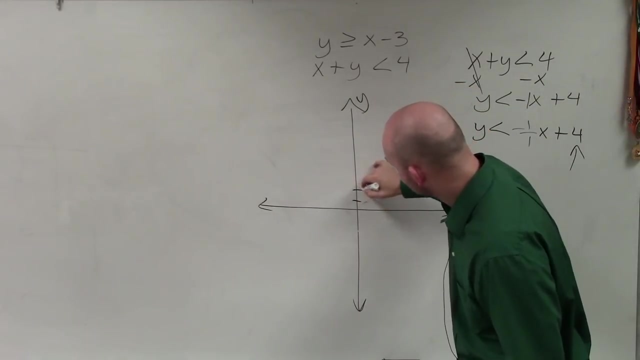 So now let's go ahead and graph it. So the first thing we do is plot the y-intercept, because I think that's the easiest thing to do. The y-intercept, remember, is going to be your constant, So I go up positive 4 on the y-axis 1,, 2,, 3,, 4.. 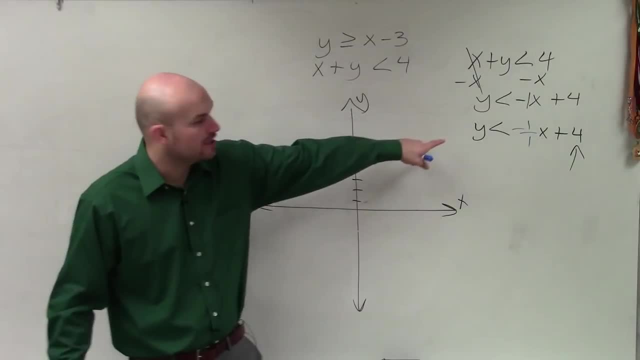 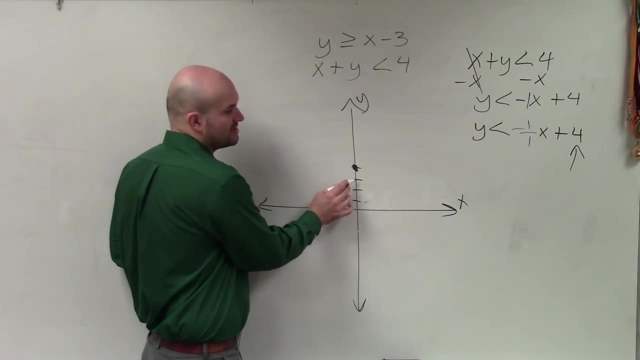 And I make a nice big dot. Then I use my slope, which says the change in the y-coordinates is negative 1, and the change in the x-coordinates is positive 1.. So since the change in the y-coordinates is negative 1,, 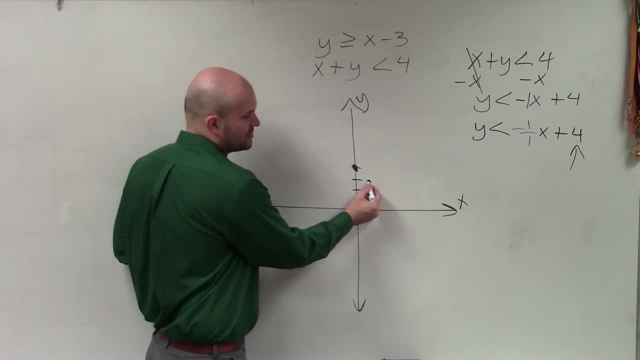 I'm going to go down, Since the change in the x-coordinates is positive 1,, I go to the right. Then I look at my inequality symbol and I notice that it is less than So. it's going to be a dashed line. 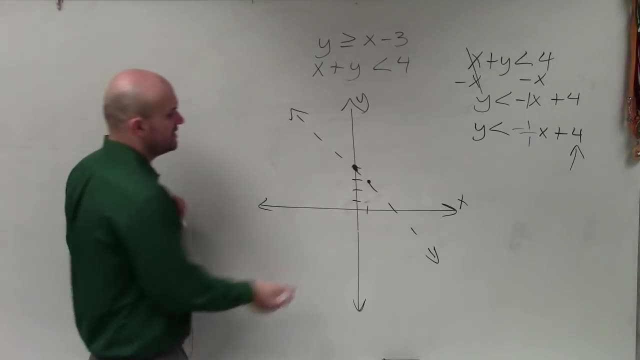 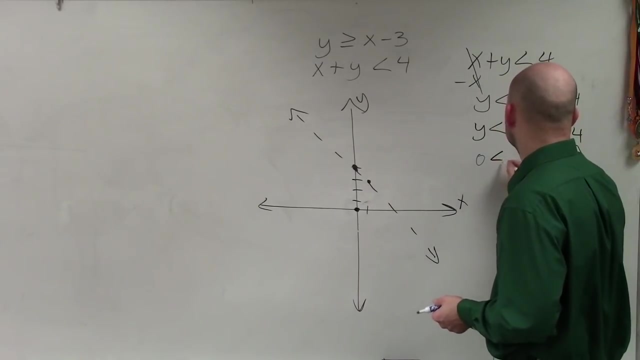 And then the last thing I'm going to do is use shading. So I'll pick 0, 0, or I test, I'll pick 0, 0, and I'll just plug in 0 in for x and 4, y. 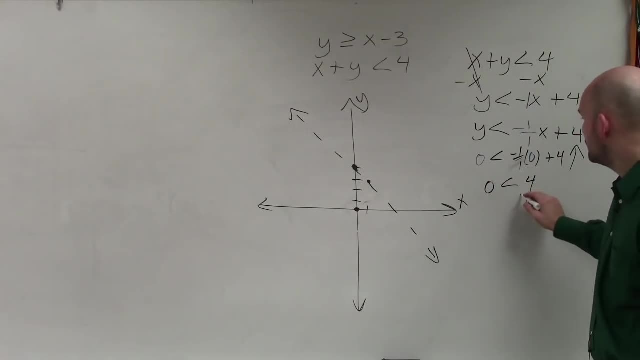 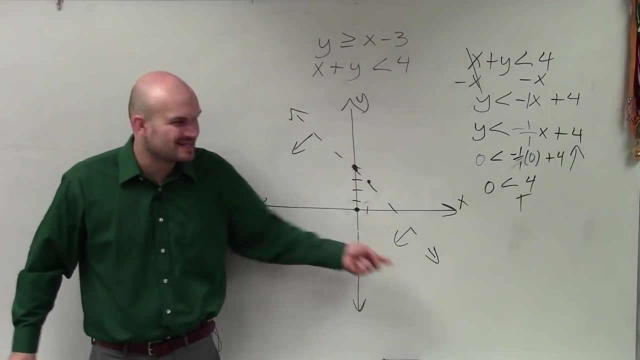 And I get 0 is less than 4, which is true. So, since that is true, I am going to shade below. However, when I have a system of two inequalities, rather than graphing all the lines, I just like to use arrows.